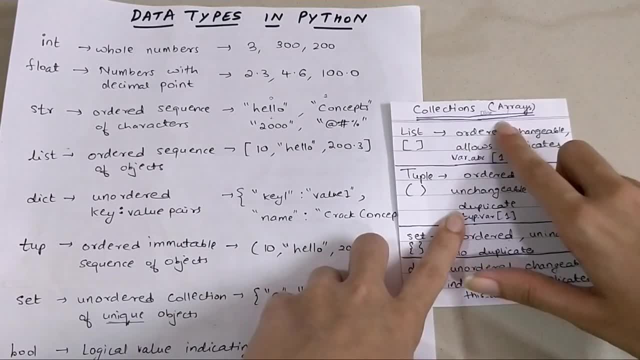 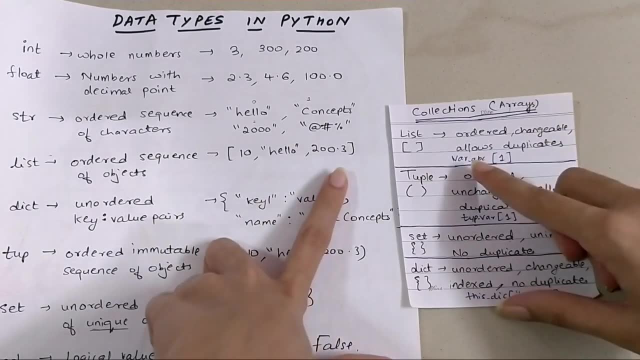 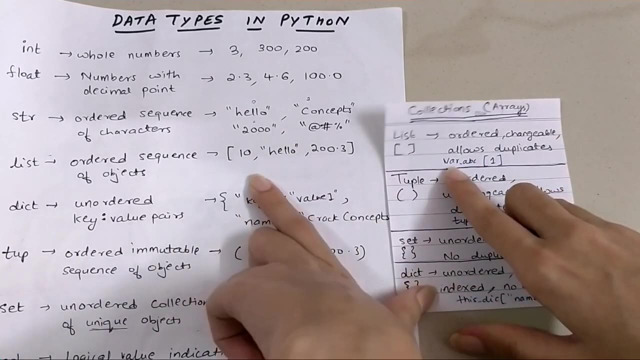 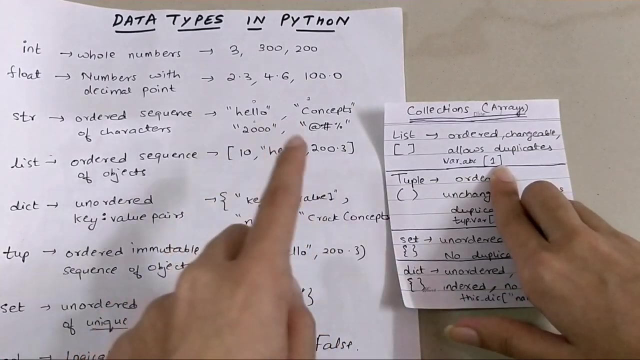 Okay, now by ordered. what does it mean by ordered? Now? now the list has these values: 10,. hello, 200.3.. What I mean by ordered is when you, when you use the index, and suppose this list has a name, var underscore abc, and when I write var underscore abc, square brackets 1, I am, I am going to print. basically, this thing is going to print the value at first: index. 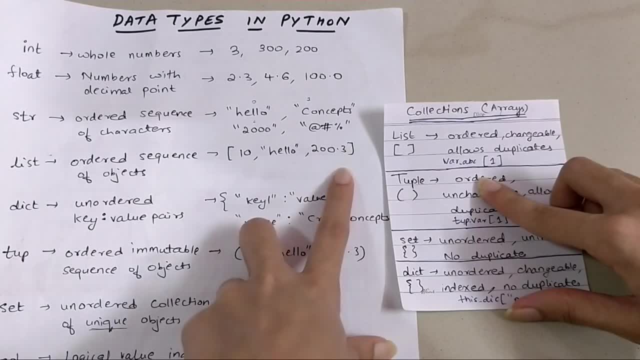 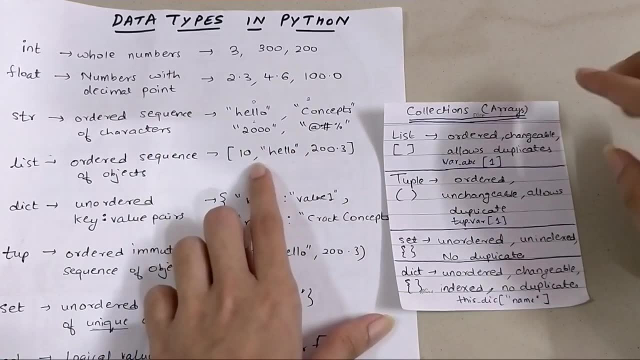 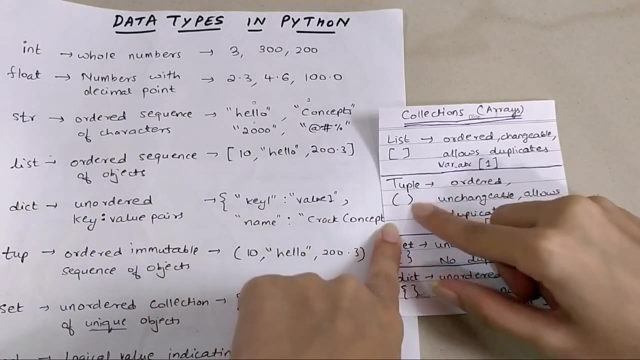 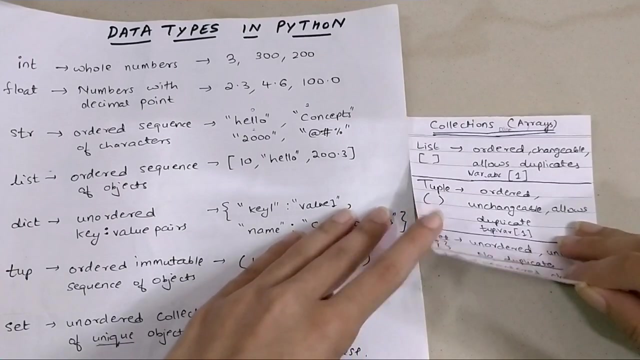 So this is your 0, 0th index. this is your first index. this is the second index, second index, So it will print hello. So ordered means they will be ordered. Okay now the second one is a tuple. Tuple is declared in in. tuples are declared in circular brackets. So tuples are again ordered, but they are unchangeable. You cannot change the values and it allows duplicates. 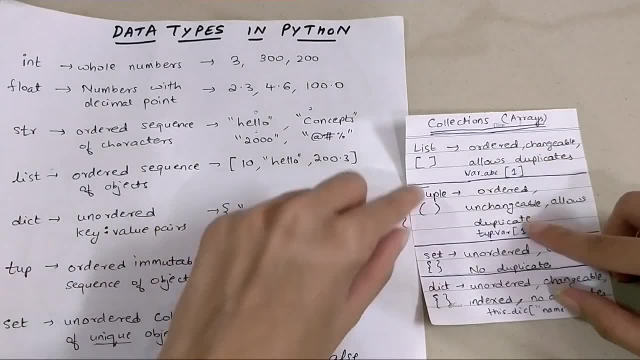 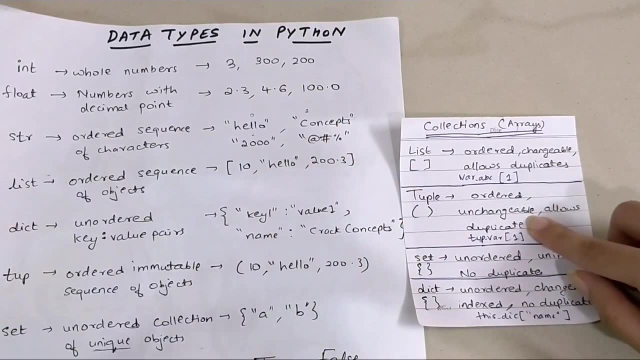 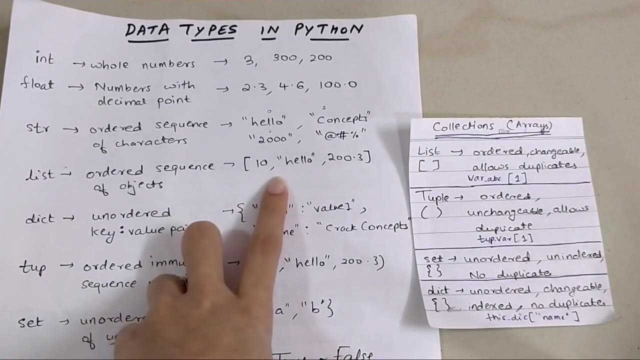 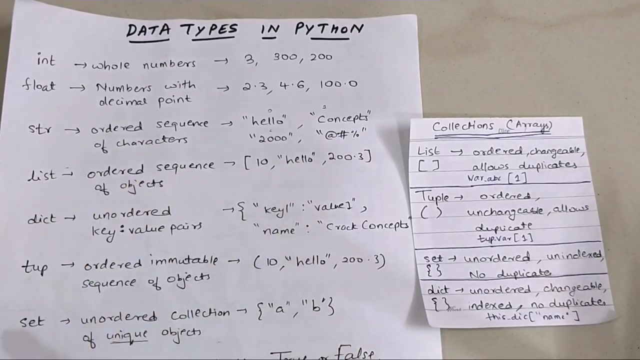 So it is very much similar to list, but the only difference is that list- list is declared in square brackets, this is declared in circular brackets and list is changeable and tuple is unchangeable. Now, what do I mean by unchangeable? Now, when you have a list, as you can see, over a list, you can change it, you can append a value, you can change a value. you can change the value at 0th index to some other value. you can do that. But in case of tuple, you cannot. Once you have declared it, it is declared. You cannot change it. You cannot append a value. 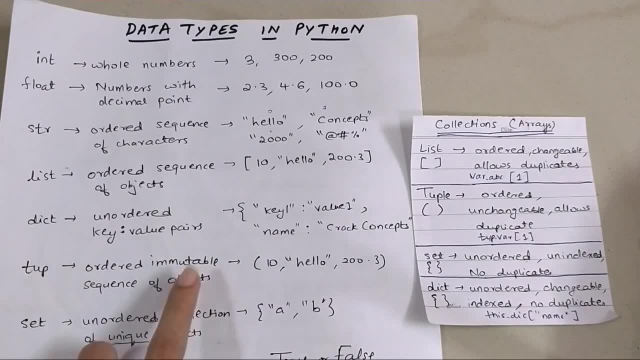 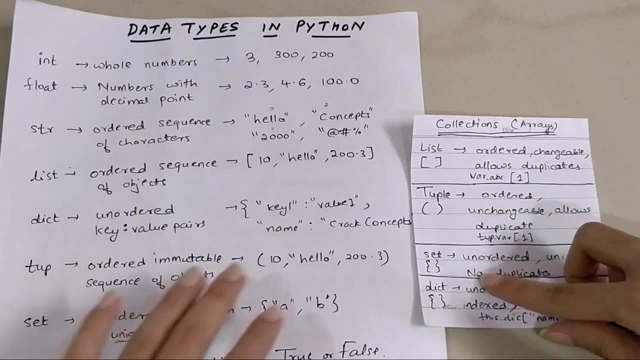 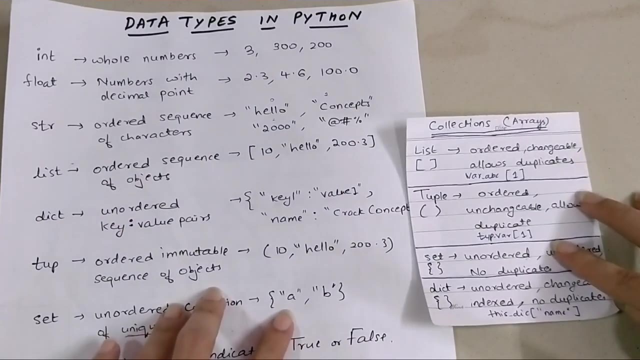 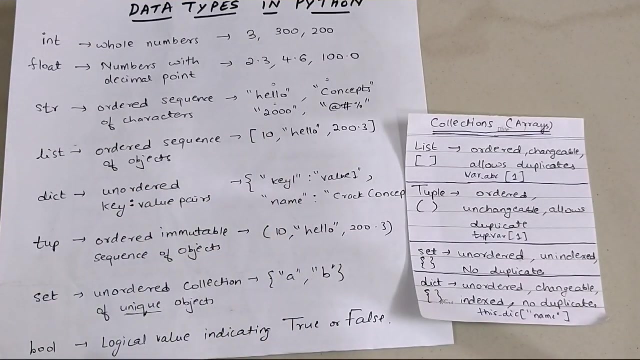 You cannot remove a value. It is not changeable. It is ordered, immutable sequence of objects. Immutable means it cannot be changed. So I hope list and tuple is clear. Now let's see set. Now what is set? Set is unordered, unindexed and it allows no duplicates. So, as you can see an example over here, it has a and b and you cannot have duplicates In case of list or dictionary or tuple- sorry, not dictionary. In case of list and tuples, you can have duplicates.